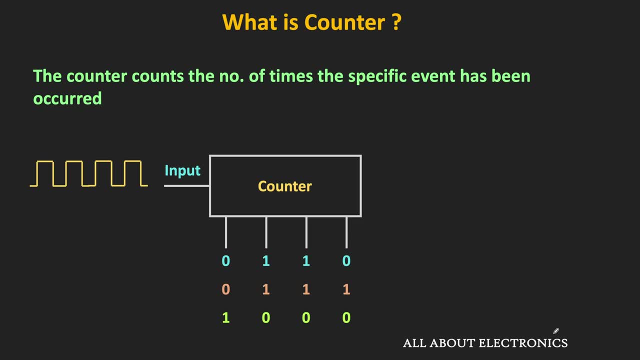 in the any other sequence. I have set a certain類 de calibrations. I can just break out the Binary sequence, then I can go into every other sequence. the counter changes in the binary number sequence, then it is known as the binary counter. 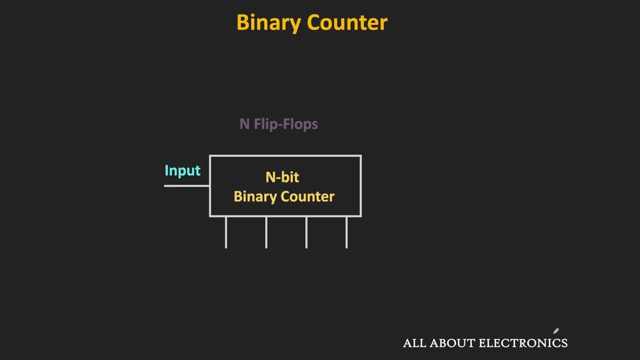 So if we have a n-bit binary counter, then it consists of n flip-flops And starting from the 0, this counter can count up to 2 to the power n-1.. For example, if we have a 4-bit binary counter, then it will have 4 flip-flops inside the 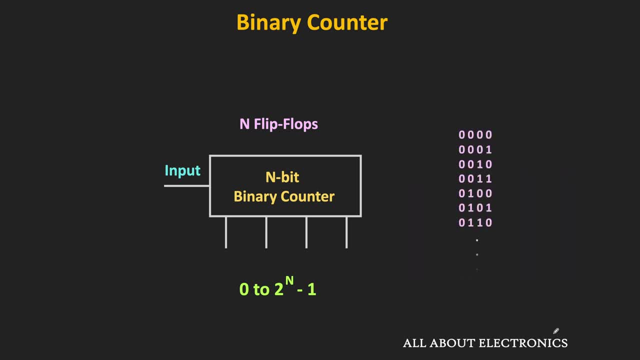 counter And it can count from 0 to 15.. So if the count of the counter goes from 0000 to 1111, then that counter is known as the up counter. But if it counts in the downward direction, that is, from 1111 to 0000, then such counter 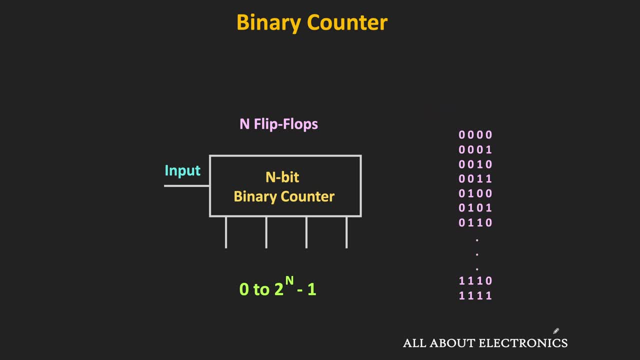 is known as the binary down counter, So in the upcoming videos we will learn about it in detail. So, as you can see over here, the output of the counter is binary 1s and 0s. So to read this count we also need some data. 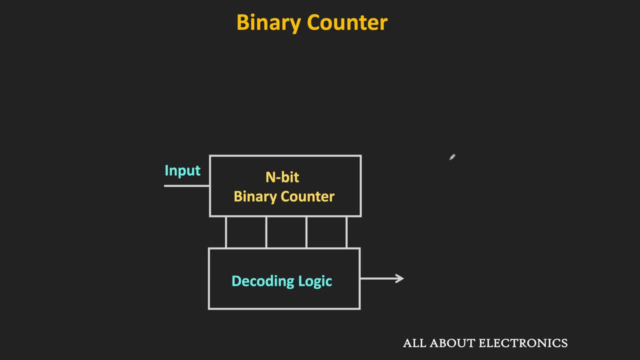 So let's look at the decoding logic And with the help of this decoding logic we can read the output of the counter. That means each counter also requires the decoding logic And with the help of the decoding logic we can know that when the counter has reached. 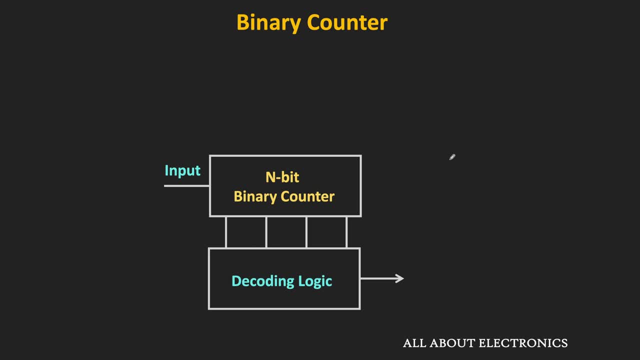 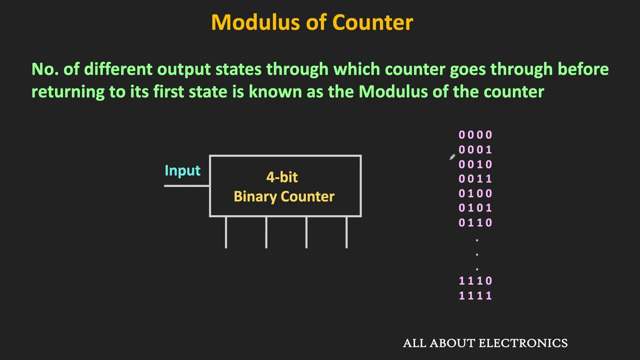 the specific count. Now, when we are talking about the counters, then we should also know what is known as the modulus of the counter. So the modulus of the counter is the number of different output states of the counter through which the counter goes Before returning to its first state. 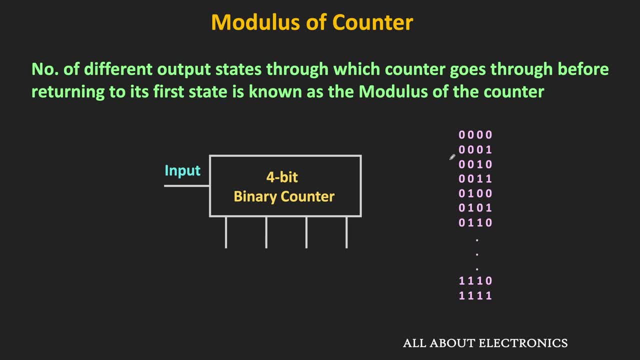 So if we take the 4-bit binary counter, then it will go from 0 to 15.. Or in the binary it will go from 0000 to 1111.. And once it reaches the 1111, then once again it will go back to 0000.. 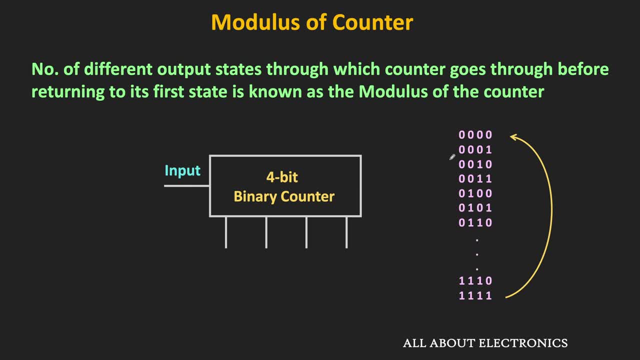 So in this case the total number of different output states of the counter is equal to 16.. So we can say that The modulus of the 4-bit binary counter Is equal to 16. Or in other words, it is the mod 16 counter. 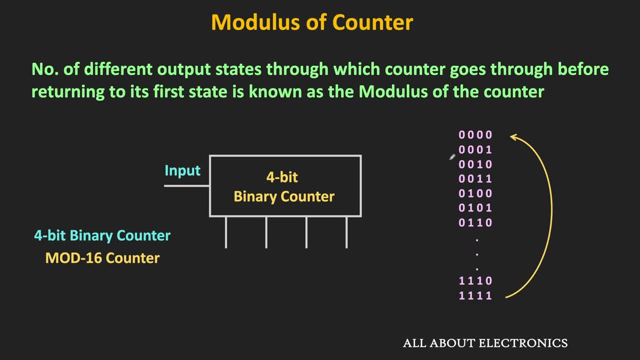 Now, sometimes the counter does not utilize all the different possible output states And in such case the modulus of the counter can be less than the maximum possible value. For example, if we take the any 4-bit counter, then the maximum possible value of the modulus 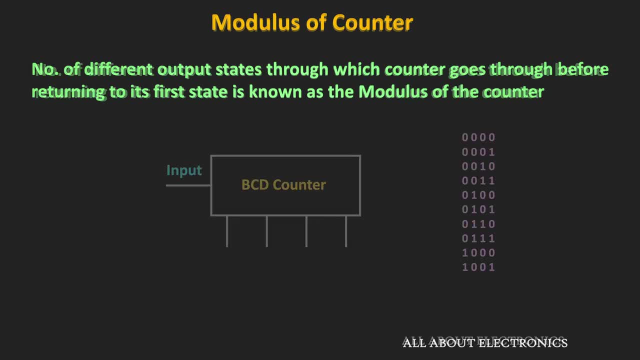 is equal to 16.. But if we see the BCD counter, Then it counts from 0000 to 1011.. That means it has the total 10 different output states, Or in other words the mod 10 counter. So although this BCD counter is the 4-bit counter, 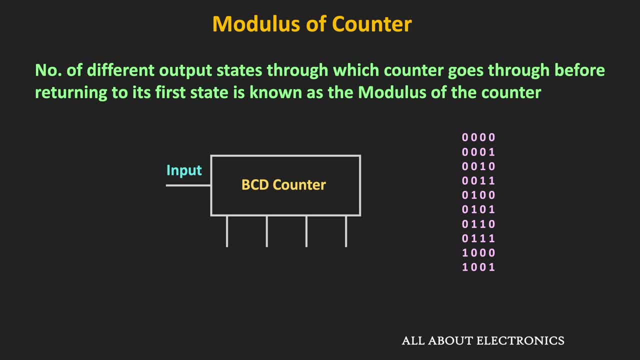 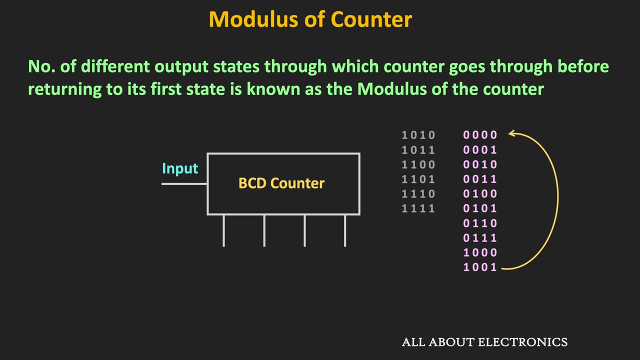 But it is not utilizing all the possible output states. So that is the brief overview about the modulus of the counter, And in the upcoming videos of the counter We will discuss more about it. So these counters are used in the many different applications. 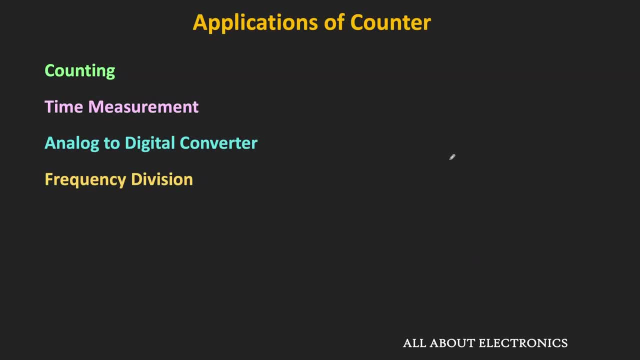 So obviously they are used in the many different models. So the first one is the DC counter And the second one is the DC counter in the counting applications, but apart from that they are also used as the timer, as well as in the time measurement applications. 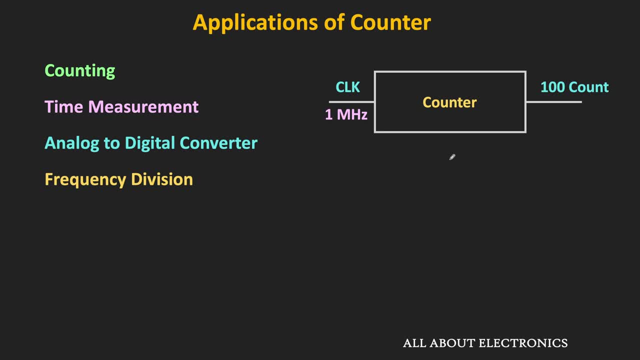 For example, if we see this counter circuit, then here the 1 MHz clock signal is applied as an input to this counter. That means here the each clock duration is equal to 1 microsecond. So let's assume that at the output of the counter the decoding logic is also connected. 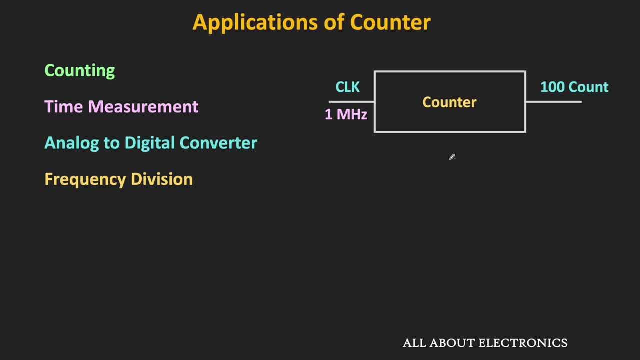 So here the decoding logic is designed in such a way that it generates the logic high when the output of the counter goes to the 100 count, and at the same time it also resets the counter to the zero. That means, with this counter we can generate the periodic pulses at every 100 microsecond. 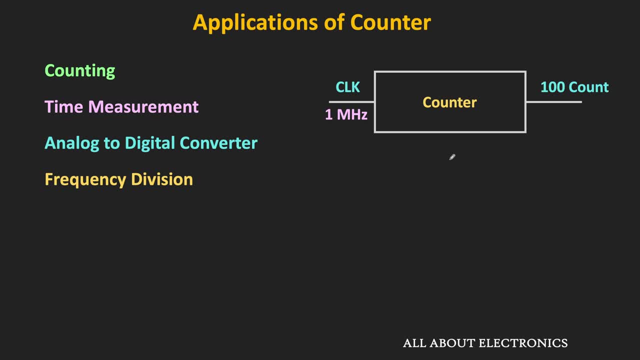 So in this way, using the counter, we can take the specific action at the predefined time. Apart from that, using this counter, if I want to measure the time duration between the two pulses, Then I can take the specific action at the predefined time. 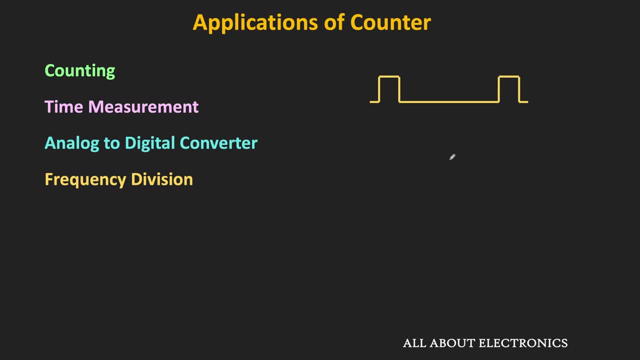 Then also we can measure that. So, with the help of the flip-flop or any other circuit, we can generate this time pulse whose duration is the difference between the two rising gauges. Now this signal can be applied to the counter with the help of the AND gate. 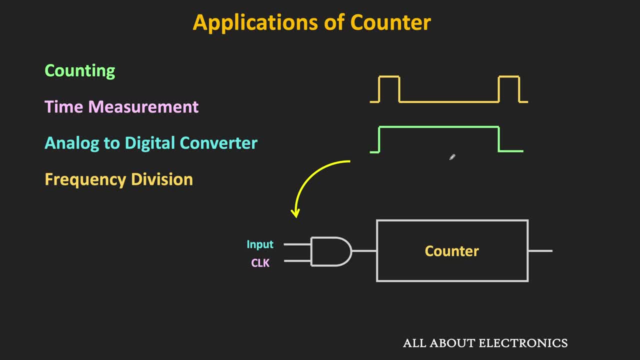 That means now, when this input signal is high, then during that time only the clock signal will be applied to the counter, And during that time only the counter will increment its count. So let's say The frequency of the clock is equal to 1 MHz. 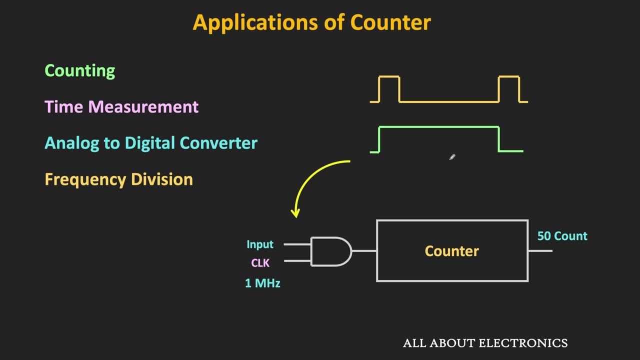 And after this duration, if the count of the counter is equal to 50,, it means that the difference between the two time pulses is equal to 50 microsecond. So in this way the counter can also be used for measurement of the time delay. 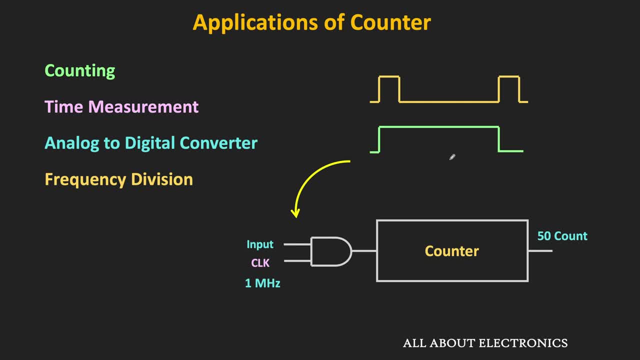 So, similarly, these counters are also a very essential part of many analog to digital converters. For example, they are an integral part of the dual slope, as well as the counter type ADCs. So these are the few applications of the counter. Now, typically, the counters can be categorized in the two types: 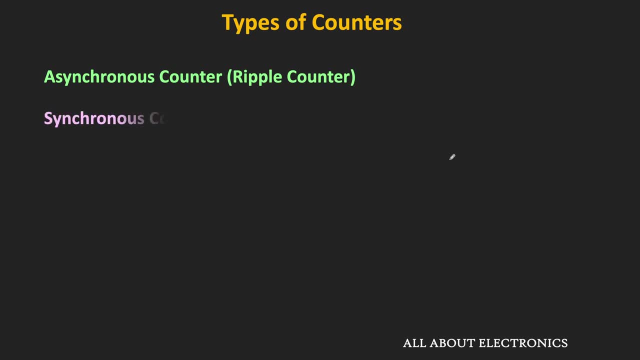 That is asynchronous or the ripple counter, and the second is the synchronous counter. So in the asynchronous counter all the flip-flops in the counter does not receive the clock at the same time. So, as shown below, only one flip-flop in the counter receives the clock and then the output. 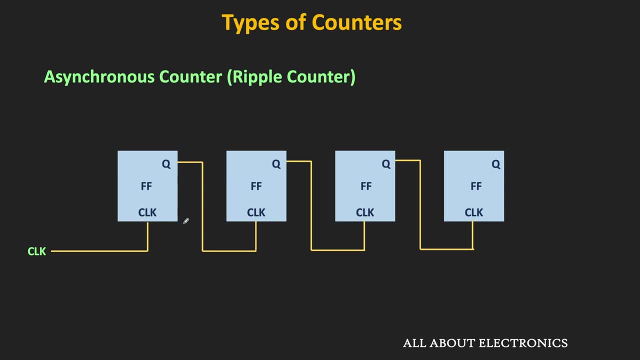 of the one flip-flop is connected to the clock itself, And the input of the next flip-flop is connected to the input of the next flip-flop, And likewise, this output of the second flip-flop is connected to the input of the next clock. 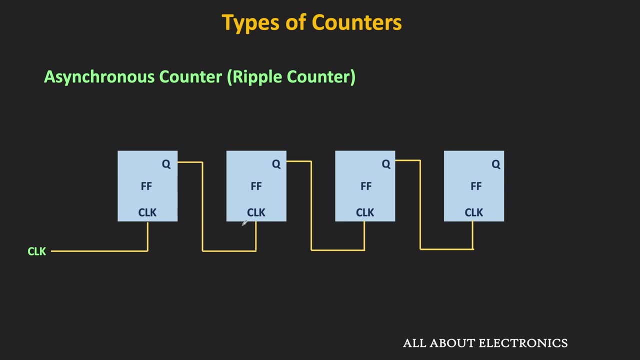 So in this way the output transition in the one flip-flop triggers the next flip-flop. So basically, here the output transition in the flip-flop acts as a clock signal for the next flip-flop. So in this way the clock signal repulse through each flip-flop before it reaches the last. 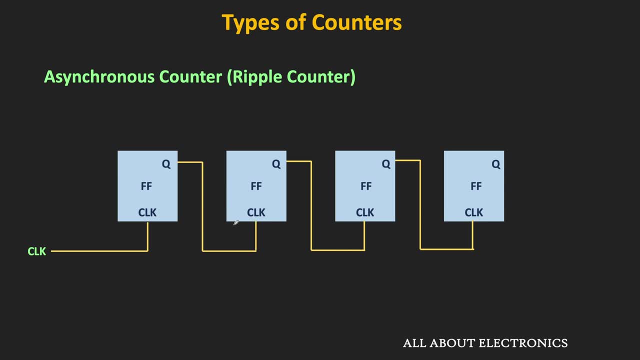 flip-flop, And that is why these counters are known as the ripple counters. So let's see how they work. So these ripple counters are relatively easy to design, but we cannot operate them at the very high speed. So that is the basic limitation of the ripple counters. 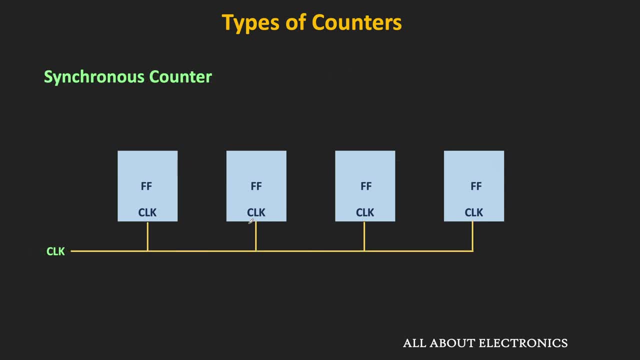 Then the second type of the counter is the synchronous counter. So in the synchronous counter all the flip-flops inside the counter receives the clock at the same time. That means in this type of counter all the flip-flops respond to the rising or the falling. 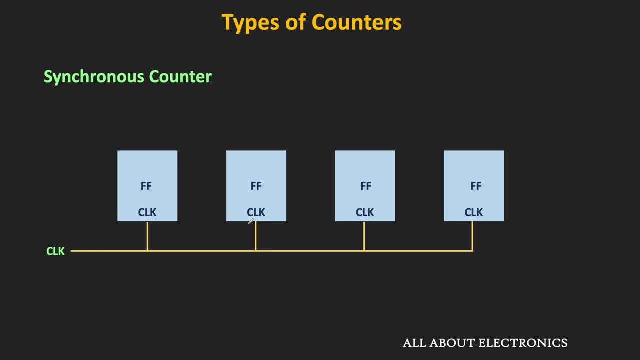 gauge of the clock at the same time And therefore they are much faster to operate, Much faster compared to the ripple counters. So in the upcoming videos we will learn about these ripple counters, as well as the different types of synchronous counters, in the detail.